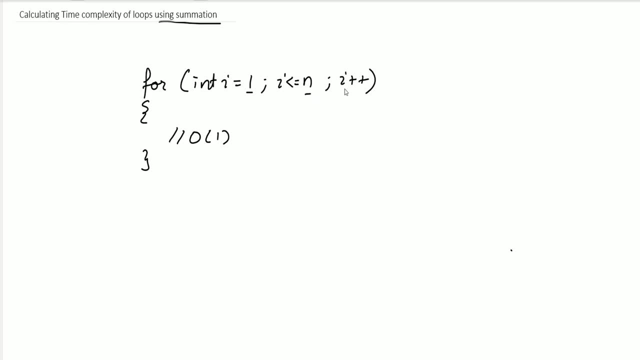 there is a loop from 1 to n in which every time we are incrementing by 1 and we are doing a constant time operation inside the loop. So what we can do is we can just write this in the form of summation: So what we are doing is this big O of 1, this constant time. 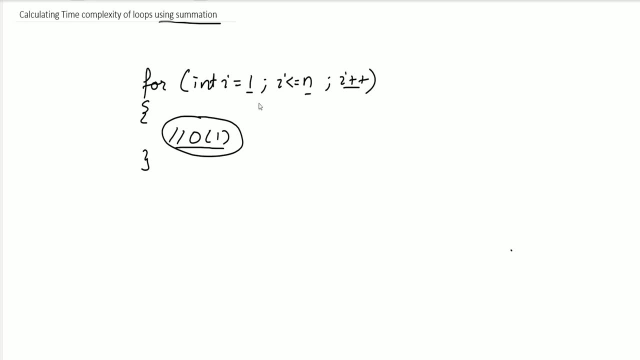 operation is happening again and again and again, from 1 to n. So we can write that summation: i equals to 1 to n, 1. This will be our time complexity. Again, we can see that this 1 we have to add, this constant time operation from 1 to n. Again and again, we have to add: 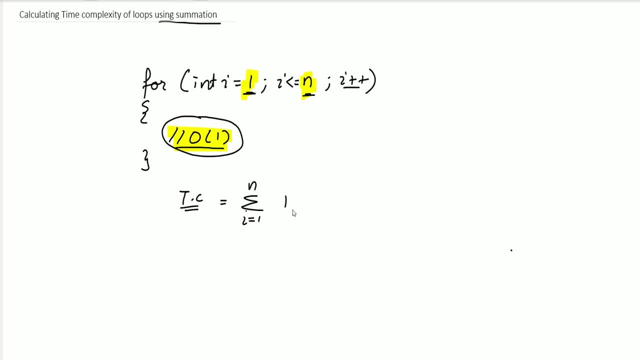 this, So we can just write: summation i equals to 1 to n and 1.. So this means, if we expand this, this will become 1 plus 1 plus 1 up to n times right, And 1 plus 1 plus 1 up. 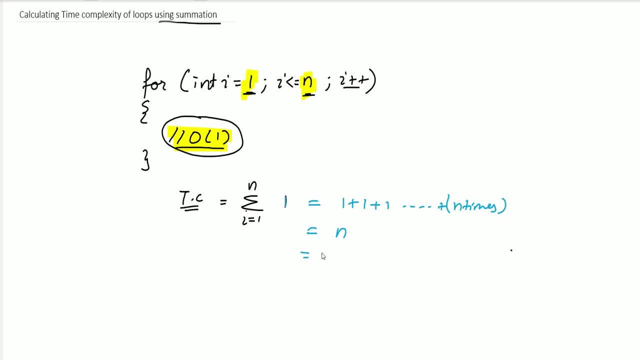 to n times. So this will be our time complexity. So this means, if we expand this, this will become n times is n. So the time complexity of this is big O of n. Let us see another example. Let us see this: For int i equals to 1, i less than equals to n, i plus equals. 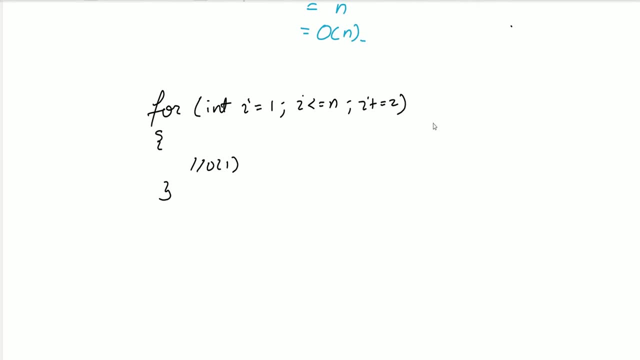 to 2.. So here we are not incrementing by 1, we are incrementing by 2.. And again we are doing big O of 1 operation here. So we can write this in the form of summation: i equals to 1 to n, 1.. 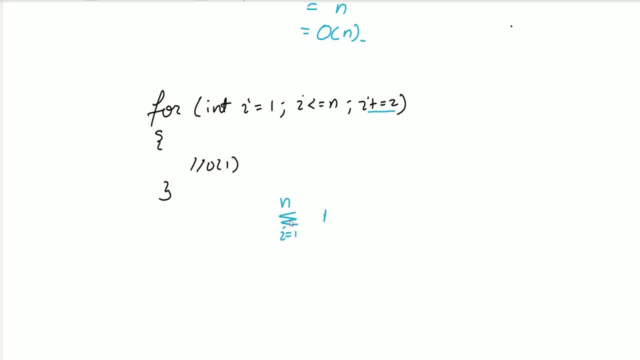 But here we are not incrementing by 1 and this summation means it increments by 1.. So what we can do is we can write: i equals to i plus 2 in the bracket here. So this is telling us that we are incrementing i every time we are incrementing it by 2.. So this: 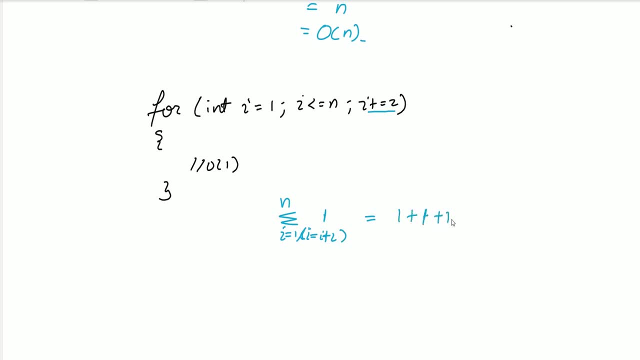 will be 1 plus 1 plus 1, up to n plus 1 by 2 times. Why n plus 1 by 2?? Let us see. So we are going from 1 to 5.. So we are going from 1 to 3 and 3 to 5.. We can see that there. 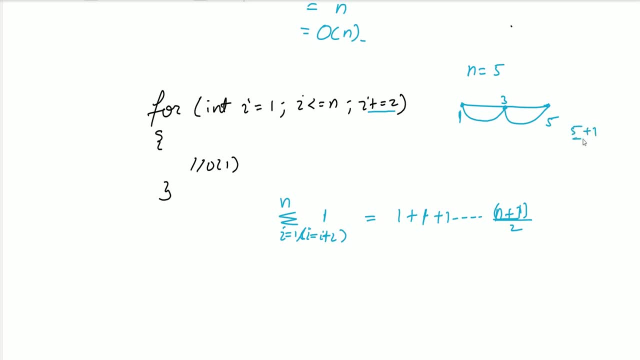 are three steps And if we see 5 plus 1 by 2 is 6 by 2 is equals to 3.. So there are three steps. If n equals to 4, then we are going from 1 to 4.. First we will go to 3. 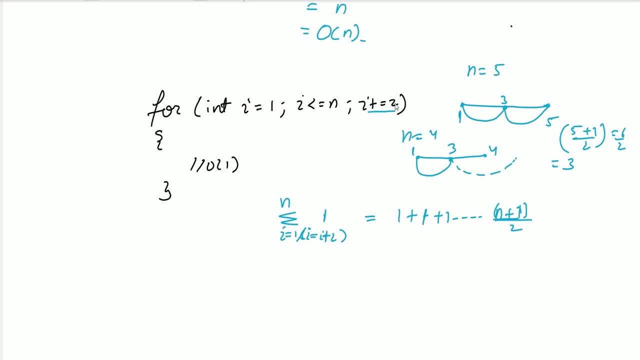 and then we will jump to 5.. But since 5 is 3, we are going from 1 to 4.. So we are going from 1 to 4.. But because n is not in the given limit, so we will not run on that. So we 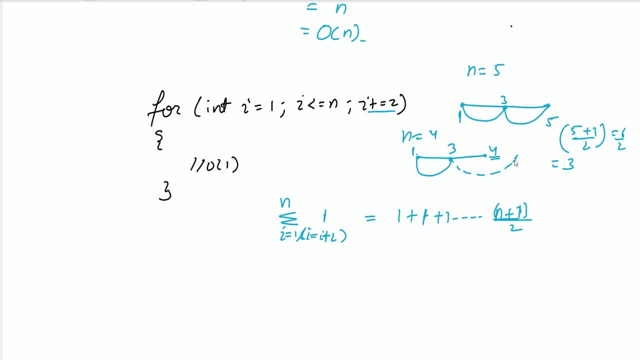 are only running 2 times. So if we see for n equals to 4, it will be 4 plus 1 by 2, which is 5 by 2, and it will be 2 only. It is 2.5, but we will take the floor, So this will. 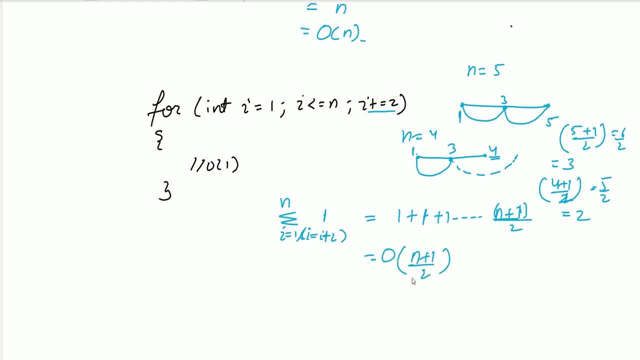 come out to be n plus 1 by 2.. So this is the time, complexity. Let us see an example in which we are doing more than we go one. Let us apply the following: Let us apply the formula. Let us apply the formula We are. 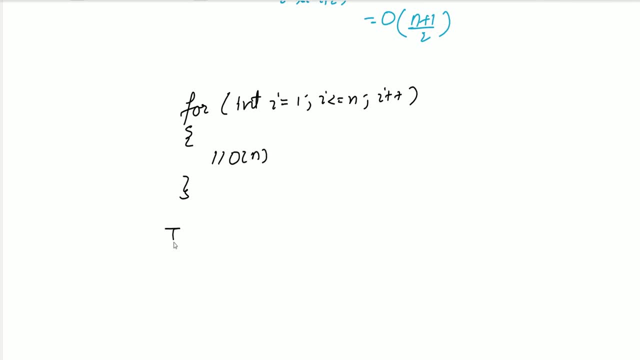 Suppose we are doing some order and operation, So the time complexity of this will be summation i equals to 1 to n, And because we are doing n work here, so here it will be n only. So now, if we see the complexity, if we expand this, this will become n plus n plus n, up to n times. 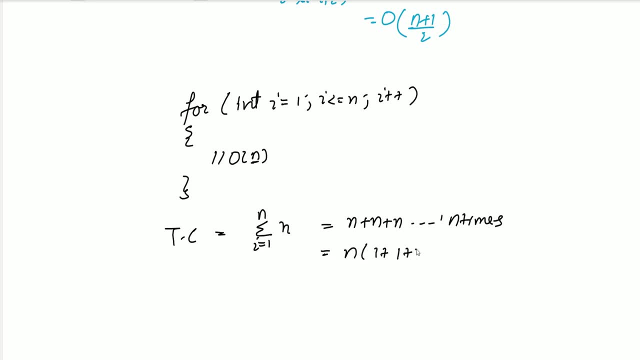 So if you take n common, it will become 1 plus 1 plus 1 up to n times, And we are seeing this. 1 plus 1 up to n times is n, So this will become n into n and order n square. 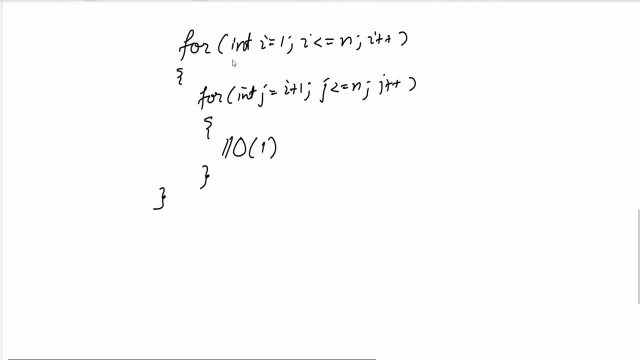 Let's take one more example. Let's see this example: for int, i equals to 1,. i less than equals to n, i plus plus. For j equals to i plus 1.. So now we are going from i plus 1 to n. 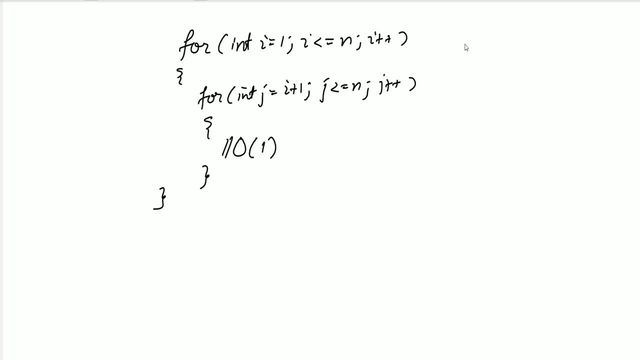 And if you remember counting this, we have to just make a table that when i is 1, then j is going from 2 to n, Like this. But here what we can do is we can just write the summation: Summation i equals to 1 to n. 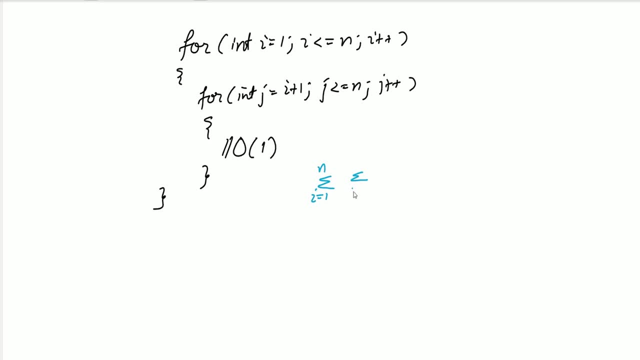 Summation, because it is nested loop. so we will have two summations: One is for i loop and one is for j loop. So j equals to i plus 1 to n And we are doing order 1 operation. Okay, so this will be our time. complexity. 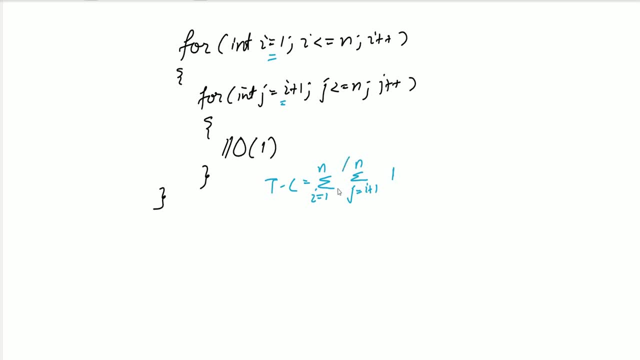 So if we find this out, what will happen? Let's first solve this summation. So this time complexity is summation i equals to 1 to n, And this will become. so we are starting from i plus 1 to n. 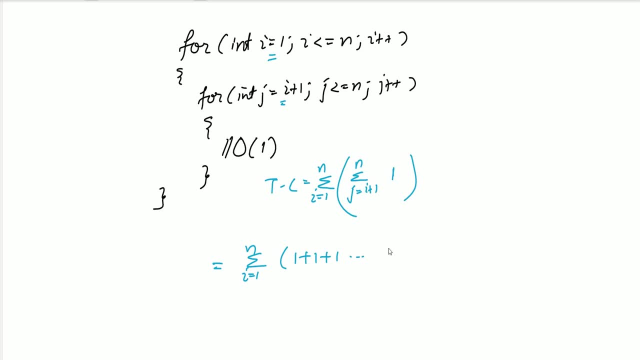 So this will become 1 plus 1 plus 1. up to how many times? So from? if we are going from 1 to n, then it is n times. Okay, how we are doing this is both lower and upper limit, So we are going from one lower limit to some upper limit. 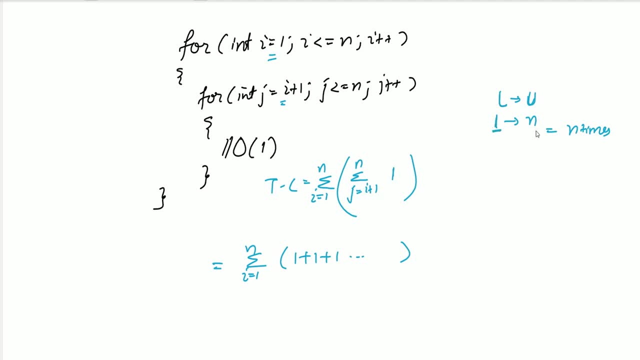 Okay, and both are included. So here 1 is also included and n is also included. So the formula is u minus l plus 1.. So if you put this in this from 1 to n, we are going from n minus 1 plus 1 equals to n times. 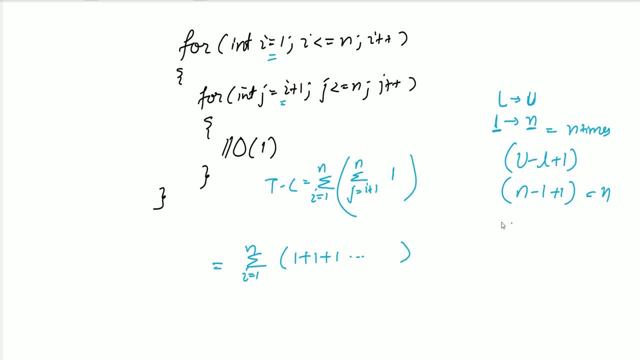 So from i plus 1 to n, what will happen? How many times we are going? The upper limit is n, the lower limit is i plus 1 and then plus 1.. So this will become n minus i minus 1.. 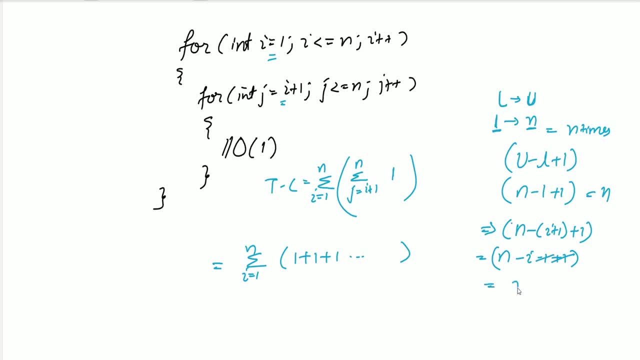 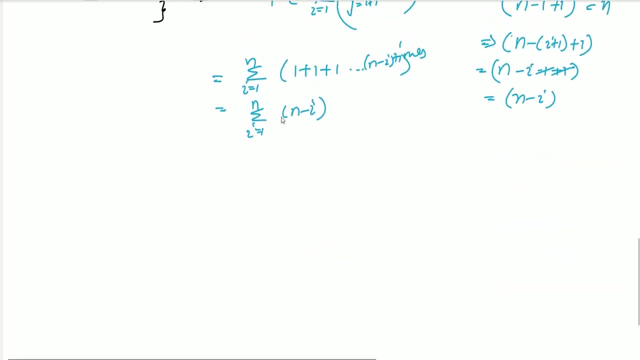 Okay. So if you remove this, this will become n minus i, So this will be n minus i times. Okay, and 1 plus 1 n minus i times is n minus i, So this will become n minus i. Now we can do summation on these. 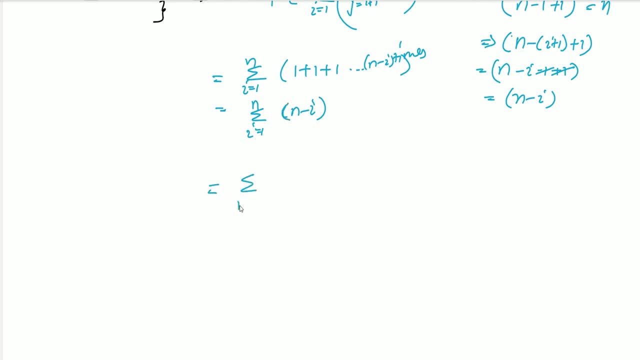 We can just divide this summation, This will become summation i equals to 1 to n n minus summation i equals to 1 to n i. Okay, And this will become, since we are adding n plus n plus n n times, so this will become n square minus. this will become 1 plus 2 plus 3 up to n. 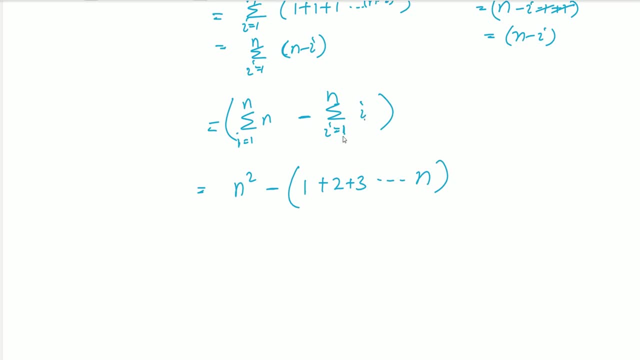 Okay, because here it is i, So we will put. when i equals to 1,, we will put 1.. When i equals to 2,, we will put 2.. When i equals to 3,, we will put 3.. 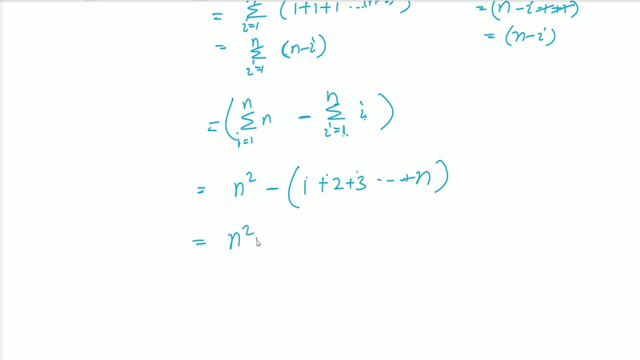 And when i is equals to n, we will put n. So this will become n. square minus sum of n natural number is n into n plus 1.. Bye, So this will become n. square minus n square plus n by 2, and this will become 2 n square minus n square minus n by 2..